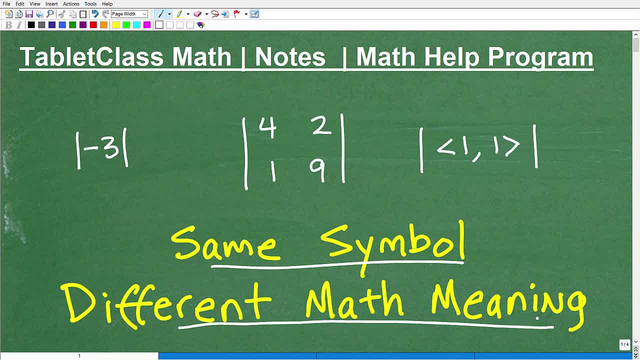 Okay, or verb, and you can have different meanings. Okay. well, in mathematics, same thing here, And I'm going to show you an example where we're using these little bars right here- okay, around this number. this has a particular meaning. Now, typically you'll learn this in like middle school, maybe like pre algebra, And then, as you continue to learn more mathematics, maybe into like algebra two, you'll use the same bars, but you'll use it in this way And this means something completely different than this. So, 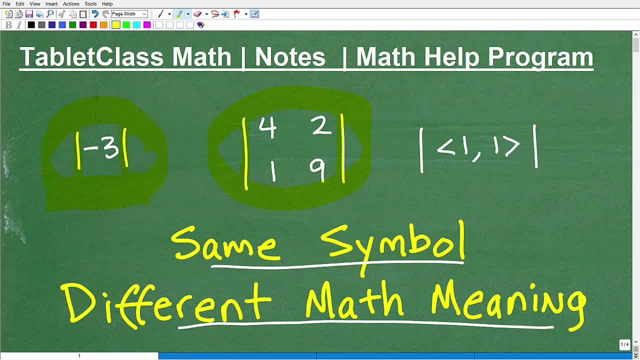 you're like, okay, wait, what's going on here? Of course, we still need to know what this means here. And then, as you continue on even further in your math education, maybe into, like, say, algebra two, trigonometry, maybe college algebra, pre calculus- certainly you'll use the same bars around something like this And this means even something different. Okay, So indeed, we could be using this, the same symbol, but it will have different meaning in mathematics. So I'm going to go ahead and use these three examples. I'm sure there's other. 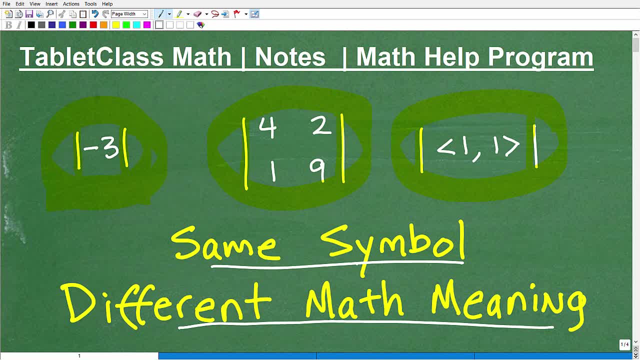 notation that you'll encounter. But these ones here in particular kind of come to mind just to, you know, make the point again, in mathematics you got to be paying attention Because you know if you're like, Oh, I understand what to do here, And when I see these bars, you know around this thing, it means do what I do over here. No, it does not, Okay. so this isn't that difficult, by the way, And I'm going to go through and explain each one of these little guys And just one second. But first let me quickly introduce myself. My name is john. I'm the founder of tablet class. 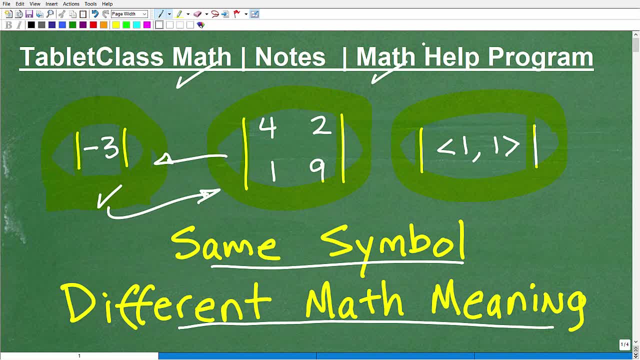 math. I'm also a middle and high school math teacher And over several years I've constructed what I like to believe is one of the best online math help programs there is. of course, I'll let you be the judge of that. If you're interested, you can check out my math help program by following the link in the description of this video. Basically, I have 100 plus different math courses, ranging from pre algebra, algebra one, geometry algebra two. I'm going to be launching pre calculus here in about about a week or so And in 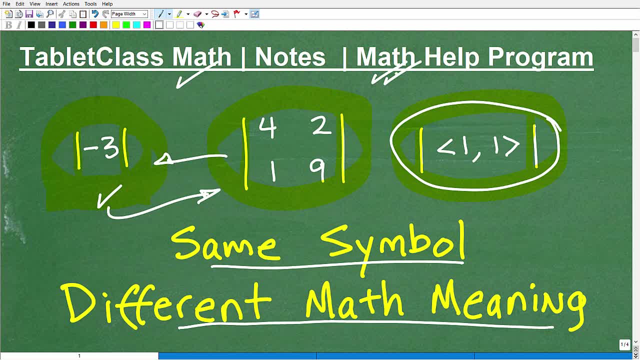 pre calculus. I get a lot into this kind of stuff, But I also have many, many courses in the area of test preparation. So if you're studying for the GED, SAT, GRE, GMAT, oh my gosh, there's so many courses out there: acuplacer or test, rather, Alex exam, CLEP exam, maybe a teacher certification exam, And there's countless other exams that people have to take for all sorts of reasons, whether you want to get into graduate school, whether you're trying to get into a particular placement to a college class. 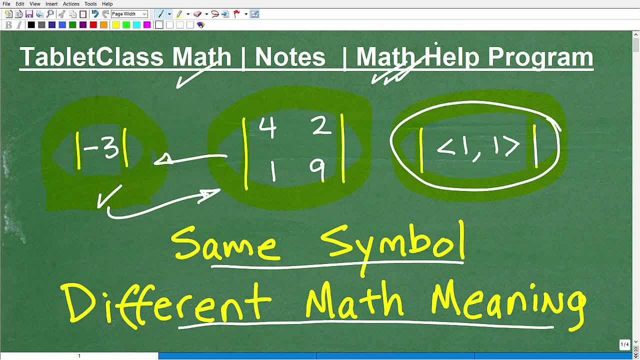 maybe you're trying to become a certified teacher, maybe trying to get into nursing school you have to take. these exams are very important and they all have math on them, Okay? so if you don't do well in the math section, you do not do well on these exams. So let me help you prepare. just go to my website and check out my full course catalog. If I do not have your exam, drop me a line in my contact form. I will help you out the best I can. I also do a lot with homeschoolers, So if you homeschool, I have a great homeschool learning system And then, obviously, help those of you that are having a tough time in 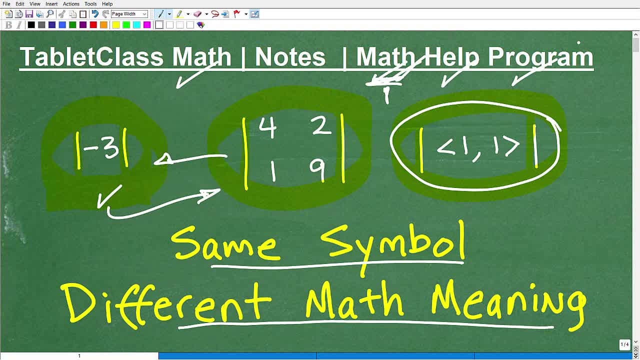 your current math courses. Now, if you're truly serious about wanting to be great at math or just pass your math course, then you got to be serious about taking excellent math notes. So I've been teaching math for decades And one thing is apparent to me: those students who take excellent notes almost always do very, very well. You know? think about it. how could you, you know, know that what's going on with this particular symbol and all the other symbology and notation you learn in mathematics, If you're not taking notes or paying attention? okay, this stuff snowballs. 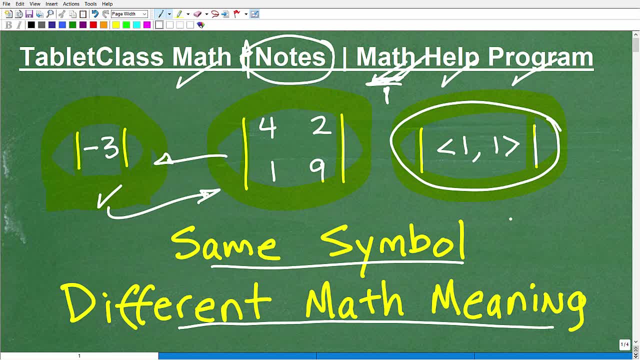 and you know there's a lot of stuff you're going to be learning, Okay. so maybe in the beginning you're like, okay, I don't need to take notes because I understand. But as you learn more and more math, it gets out of control. So you got to take great math notes And if you know, if you don't, okay, well then you know you're going to end up with grades looking like this And you know there's no need for that. Okay, you get. everyone is capable of getting at least an A. at least that's what I believe. Now, in the meantime, as you're improving your notes, you can use my notes to study, So those would include. 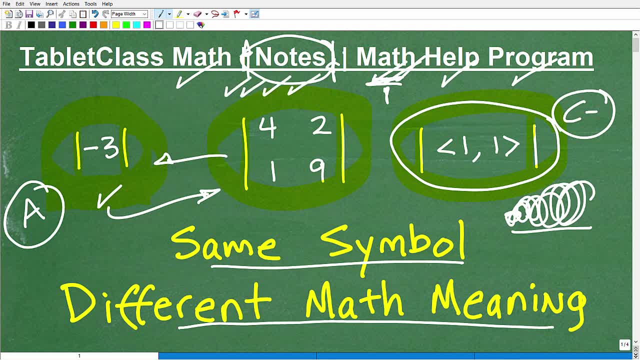 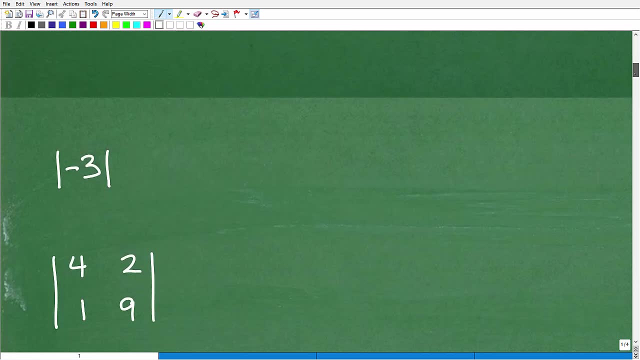 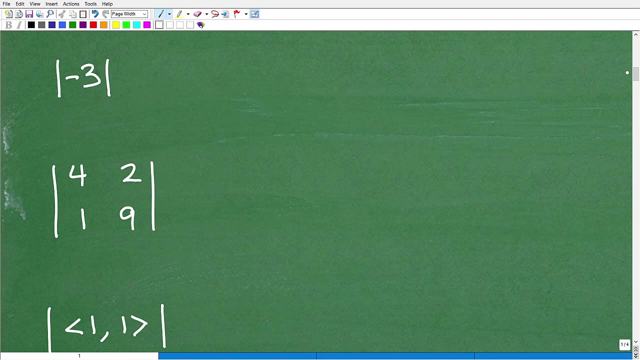 algebra- algebra one, geometry, algebra two and trigonometry. you can find the links to those notes in the description of this video as well. Okay, so let's talk about these symbols. And you know, the whole point of this video is to kind of reinforce that mathematics is a language. Okay, it's no different than learning English, Spanish. whatever the case is, it truly is a language. Okay, so we're going to go through each one of these guys. I'm not going to turn this into a full lesson, But first of all I'm going to ask you: 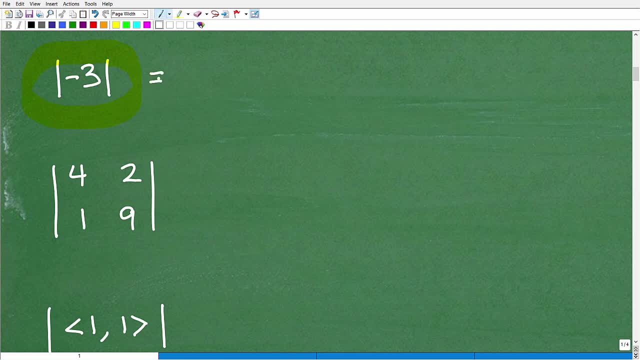 okay, what do you think this is? I know, hopefully, if you are in any kind of math course, from pre algebra and beyond, okay, you should know what this is. And if you said, Oh, isn't this the absolute value? Well, you are right. Matter of fact, I'll give you a little bit of a smiley face and a checkmark: This is absolute value. Now, what does absolute value mean, though? Okay, well, the absolute value, most of you. first of all, let's just get the answer here. What's the absolute value negative three? Well, 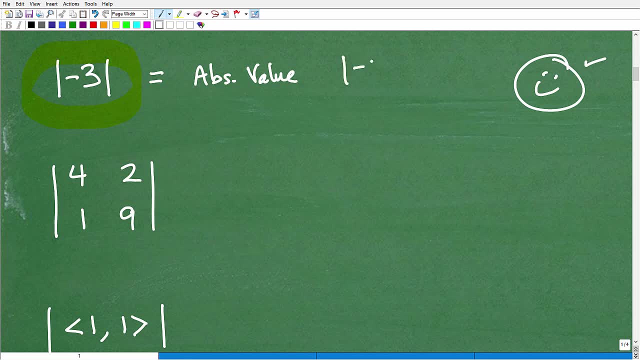 let's do this over here. Right? just a quick crash course: absolute value: negative three is three. Now, probably- oh I don't know- 70% of the students out there think that the absolute value means take this whatever. if it's a negative number, just give me the positive version of of that value. Well, this is what we call absolute value function, But really what it's asking us to do is tell us the distance a number is from negative three. okay, from zero. 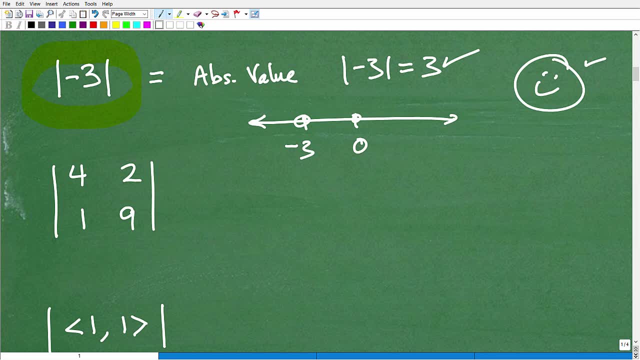 right, The distance a number is from zero is the definition of absolute value. Okay, so how far is three from zero? Well, it's three units. we measure distance in positive units. Okay, so, like you look at your tape measure or ruler, if you're measuring something- the tape measure- you don't see negative numbers here. Okay, so distance or displacement is positive. So three is three, three from zero is three units and negative three is three units. 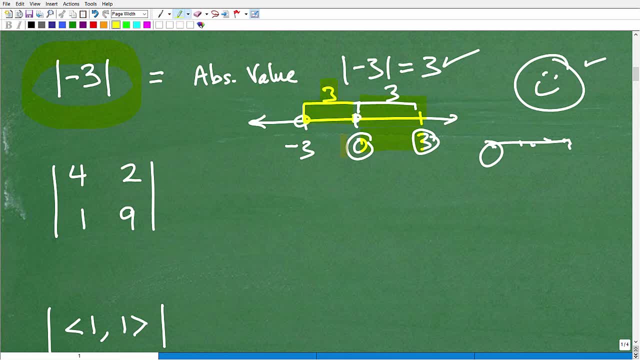 So that's the definition of this symbol. Okay, when we use it around a number, that's the absolute value. Okay, now if you didn't understand, if you actually knew this- okay, I'm pretty sure you remember this to some degree, hopefully. But if you knew this right off the bat, you're like, okay, the absolute value is a distance, a number is from zero, then that's excellent. Matter of fact, I'll throw in a couple stars, because that's very good. Okay, if you just knew the answer, that's good as well. 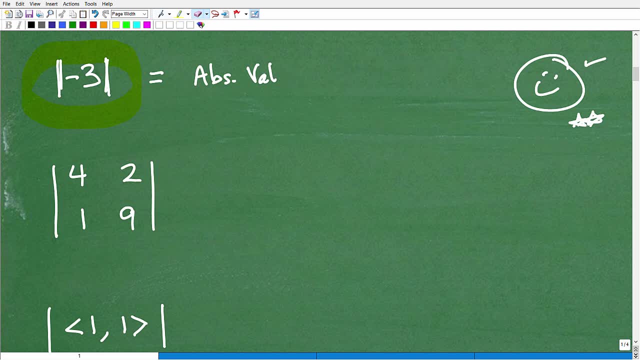 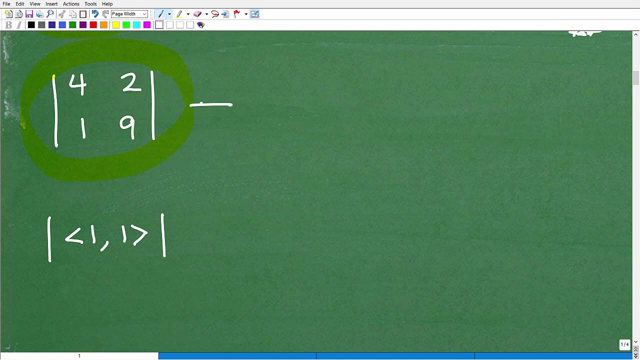 But you know, we want to know the meaning of this stuff. Alright, so we got this down here. the same, this symbol. when we use it around a number, we're talking about absolute value. Alright, now, what about this guy right here? What does this mean? Well, this is a whole different deal. Okay, this happens to be what we call the determinant, Okay, a determinant of a two by two matrix. Okay, so like, oh my goodness, what's that? Well, a matrix is a way to 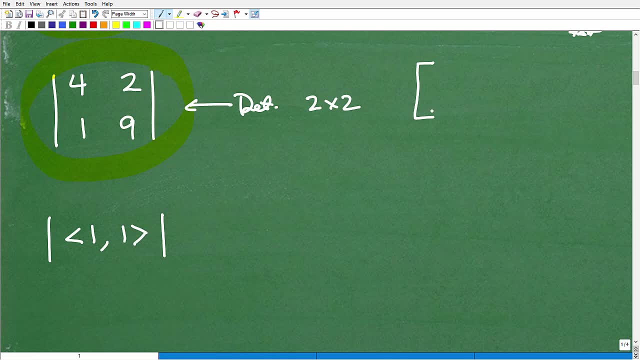 organize an array, basically organize things in a table using column rows and columns. Okay, so, like A, B, C, D, this is a matrix. Okay, so you're definitely going to be studying this in algebra, and definitely certainly in algebra to intermediate algebra, college algebra- you should have some introduction to it, And the algebra one level as well. But when we're dealing with matrices, we can do all kinds of stuff with them. you can add: 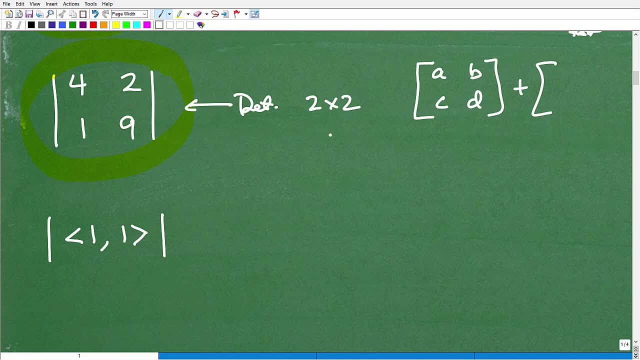 them, You can find the inverse of them. potentially, you can find the determinant, Okay, so this is what this means. Okay, we want to find the determinant of a matrix, And let me just write this right here. So we have this matrix. Okay, we measure or we define a matrix by its dimension, So that's its rows, Okay, this is its rows and this is its columns. All right, so this happens to 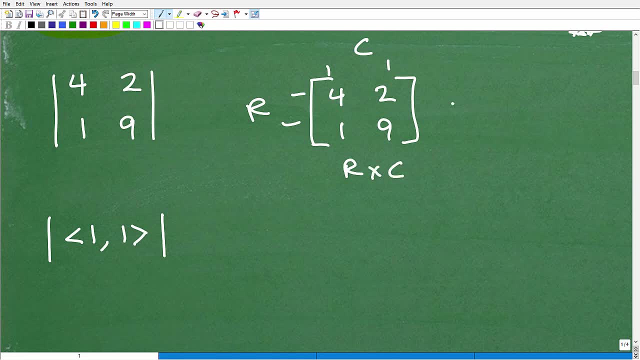 This happens to be. we define it by rows and columns, so this is a 2x2 matrix right here. Now notice this symbol, this little bracket. this is a bracket. It looks kind of like this bar, but they're different. 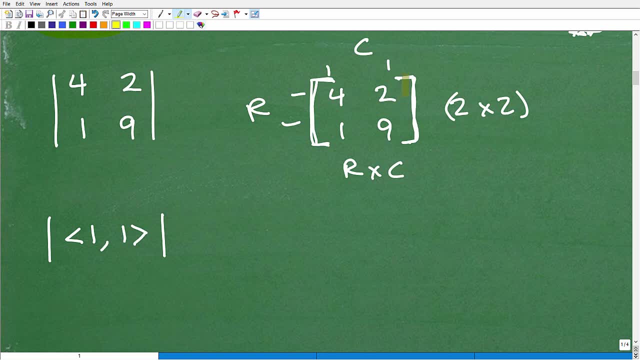 When we have this bracket, this is indicating this is a matrix, a 2x2 matrix to be specific. Now, if I want to find the determinant of this matrix, I need to put the same entries here: 4, 2, 1, 9.. 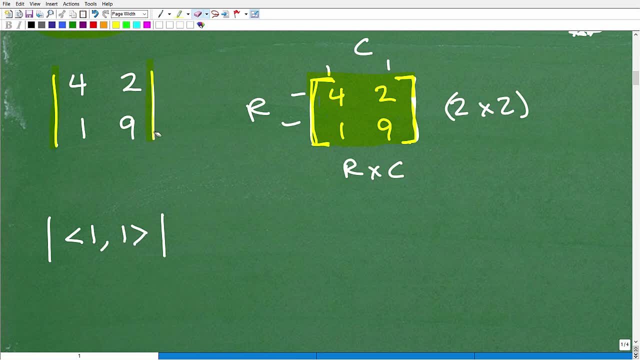 And I put these little bars around it. So this right here does not mean find the absolute value of this matrix. Now, of course, once you learn about the absolute value, you might be saying: oh, they want me to find the absolute value of all this stuff. 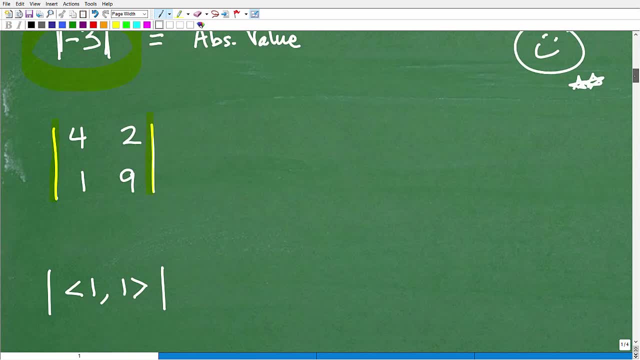 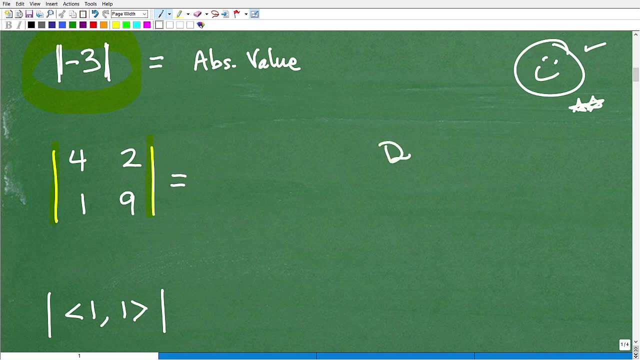 No, it does not mean that, It means find the determinant of this matrix. So you know obviously like: hey, well, how do we do this? First of all, what is the determinant of a matrix? Well, when you have a matrix again like 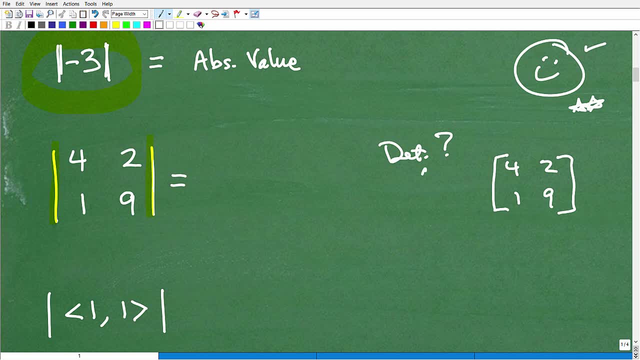 let's say you have a matrix like this. Let's say you have a matrix like this. Let's say 4, 2, 1, 9.. The determinant is just a number. okay, It's a number that is associated with every matrix. okay. 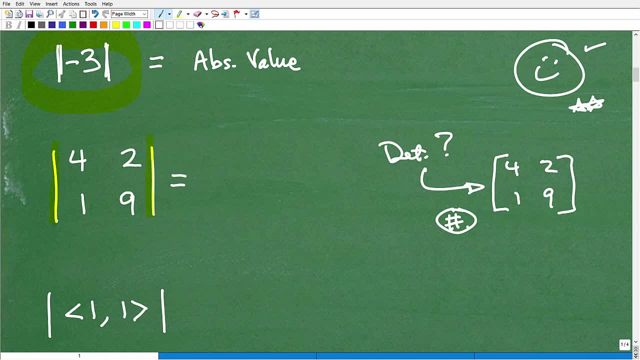 Every square matrix, to be precise, And it has value to us. okay, But the actual value determinant really doesn't mean anything particular. So when we're finding the determinant of a 2x2 matrix, it's quite easy: All we need to do is multiply these numbers first. 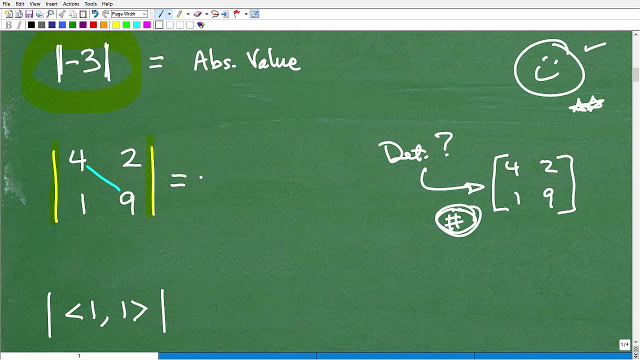 So 4x2.. 4x9.. If my arithmetic is doing pretty good today, that's 36.. And then we're going to subtract it by 1x2.. And that, of course, is 2.. So the determinant of this matrix is 34.. 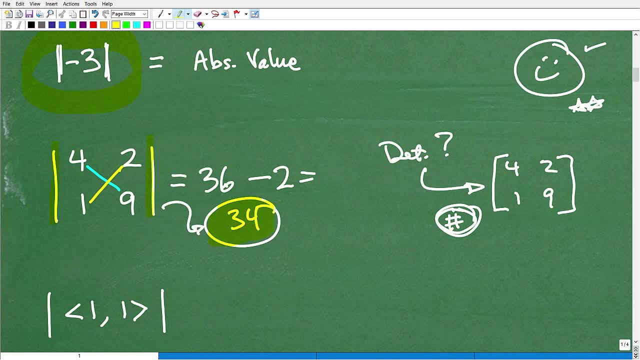 Okay, so that's the answer. What does that number mean? 34 in and of itself, Nothing special, okay. However, we can do things with that value. okay, with the determinant of a matrix to figure out other cool problems. 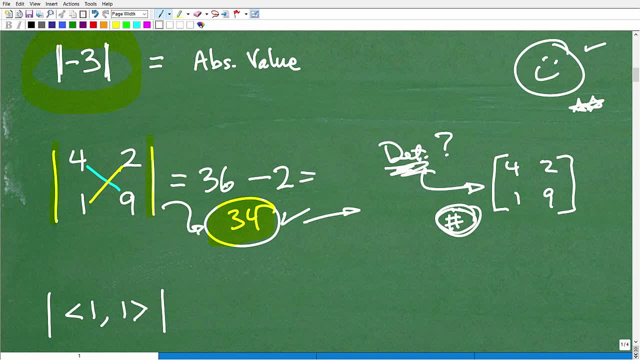 It's extremely important, by the way, to be able to find the determinant of a matrix. Now, a 2x2 matrix is quite easy. However, I can have all kinds of determinant problems. There's things that look like this: 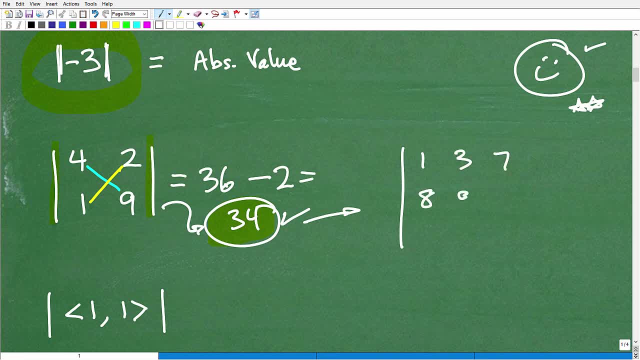 Let me just do something real quick: 8, 9.. I'm just making stuff up: 1, negative 6.. So here I'm finding the determinant. I want to find the determinant of a 3x3 matrix. okay, 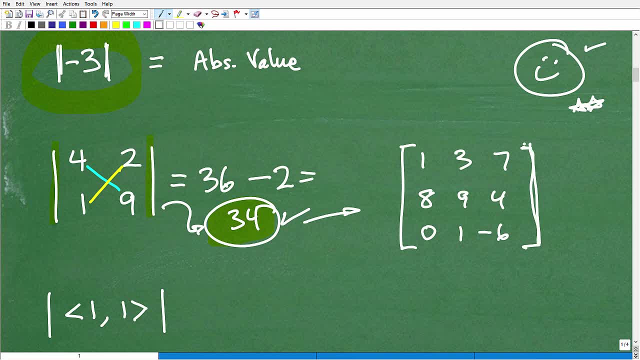 A matrix. that was this. Oh sorry, Here's the matrix. okay, And I want to find the determinant of that matrix okay, So I would use the notation, these little bars like: so. Now, how I do this is much more involved than how I did this problem, okay. 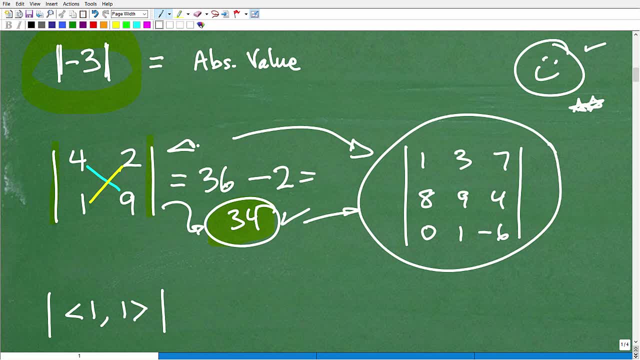 So again, you know when you're thinking about math, all this stuff I talk about note-taking and everything else. if you're watching this video, I'm assuming you're interested in mathematics and you're likely a student. So hey, you know, I'm going to teach you a little bit of math. 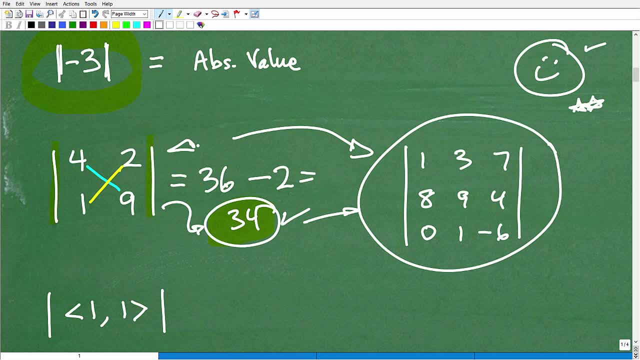 and I'm going to really emphasize the things that are going to make you successful in mathematics. okay, And I know you don't want to hear you know, oh, you know, take good notes. Nobody wants to hear that kind of you know. 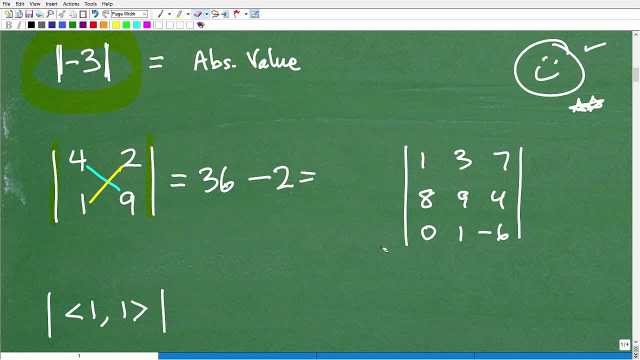 the stuff you got to do on a daily basis, the hard stuff. Well, unfortunately, it's true, There's no shortcuts. There's just too much stuff to learn in mathematics. You got to be paying attention, Okay. So these little bars right here mean the determinant of a matrix when we're using it this way. 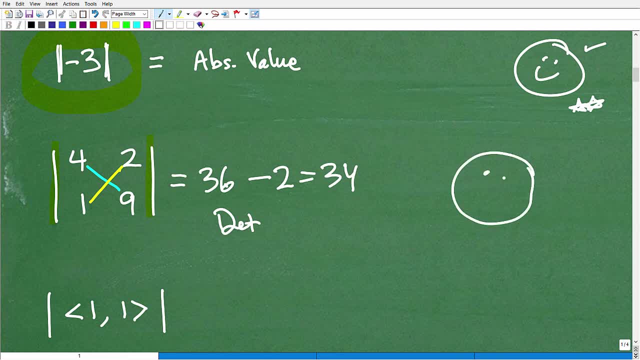 And if you knew that I must give you a bigger smiley face Right here And a matter of fact, I'll give you two, three, I'll give you three check marks and three stars. That's pretty good, Okay. 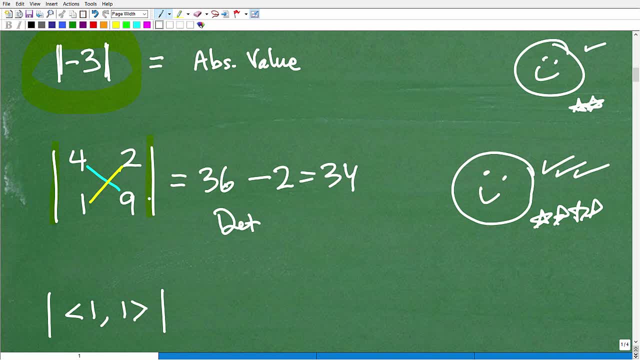 Now again, if you haven't taken a course where you've learned about matrices, you're going to see this, Okay, So when you do see this, don't confuse this as absolute value, All right, So let's finish up with this last little example. 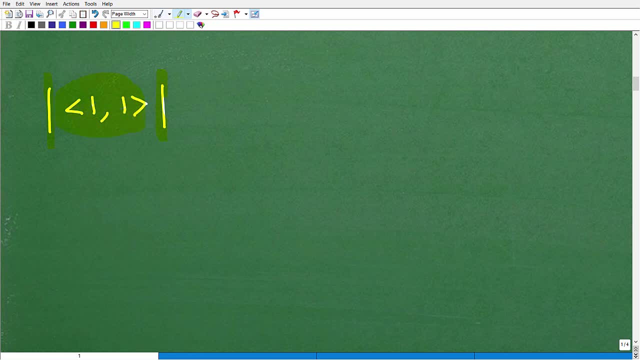 All right, So same bars again. But first of all, what is this right here? Okay, You're like, hmm, I don't even know what this is. What is that? Well, this symbol right here happens to represent a vector. 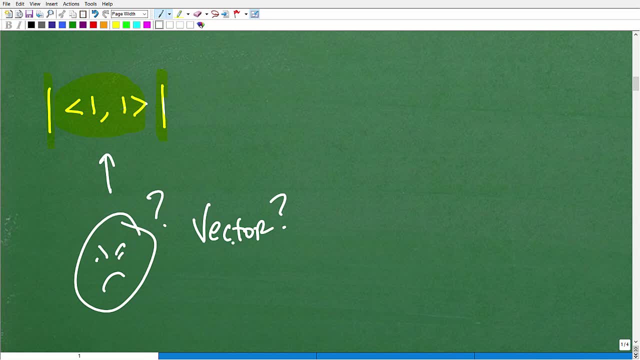 Okay, A vector. Oh, my goodness. What's a vector? Well, a vector is something that represents both magnitude and direction. So, for example, let's say: here's my lovely little airplane. Okay, I'm flying my airplane. 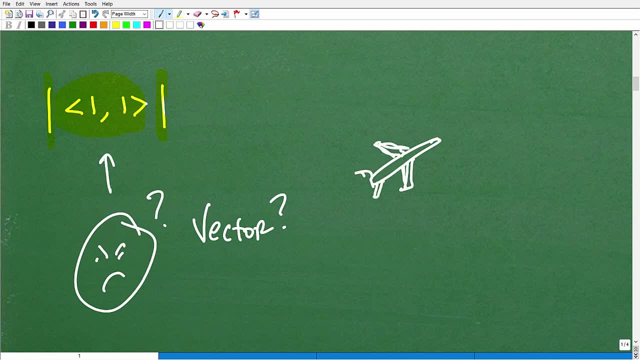 That's a terrible wink. All right, It's a little bit better. So here's my airplane and it's going, let's say, 400 miles per hour. Okay, So this is just magnitude, but vectors represent both magnitude and direction. 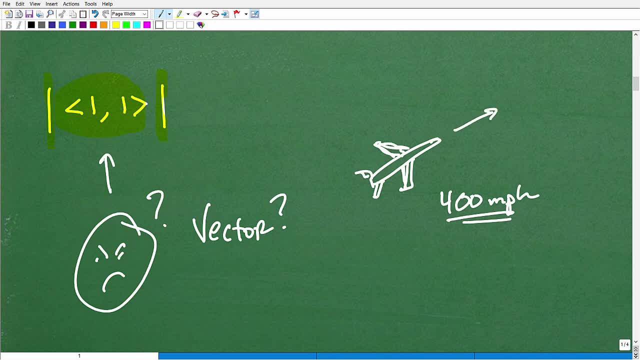 So let's say, this airplane is going 400 miles per hour on a course of 045 degrees. Okay, So when you have both magnitude and direction, you have what we call a vector. All right, Now this right here is asking us, this bar right here is asking us to find the magnitude of this particular vector. 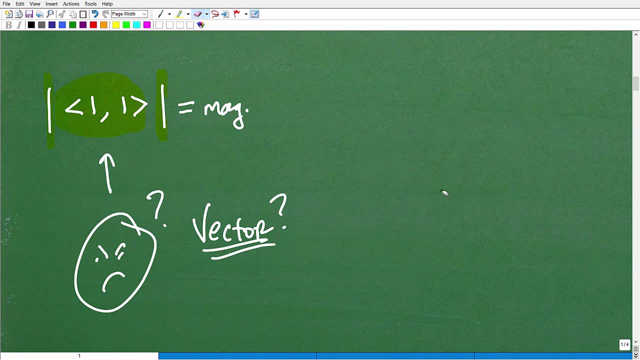 Interesting. So how do we do that? Well, effectively you can write vectors in all kinds of different ways If you don't even know what a vector is. I just gave you a quick 30-second crash course on a vector. But basically what we can do here is we're saying: okay, this little thing right here. this notation means our vector is at, it starts at 0, 0, and we go 1 and 1.. 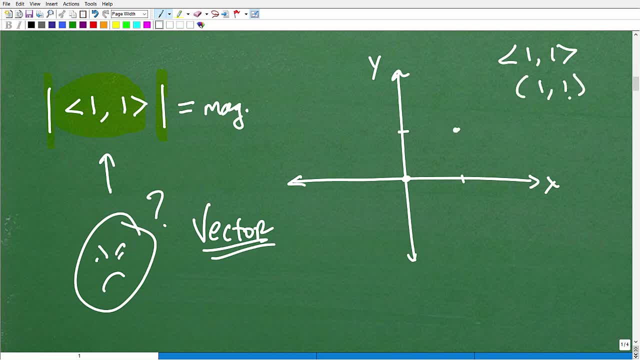 Just think of this basically as an order pair, Like a coordinate: x, y, point at 1, 1.. Okay, So there's the point 1, 1.. This is the vector And our vector is: we represent vectors as little arrows. 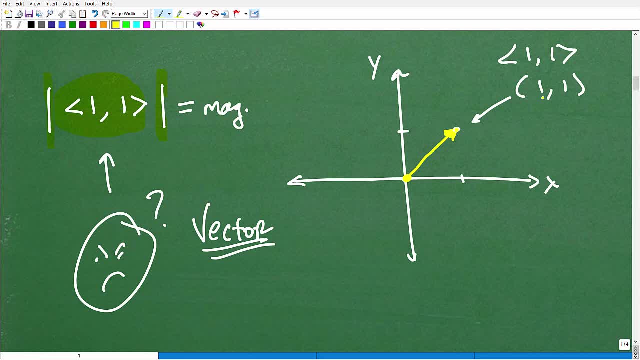 Okay, So the tip of that arrow ends at 1, 1.. Now what I want to do is find the length of that vector. That is the magnitude. Okay, That represents the magnitude of a vector. Of course, you've got to study vectors at a further level. 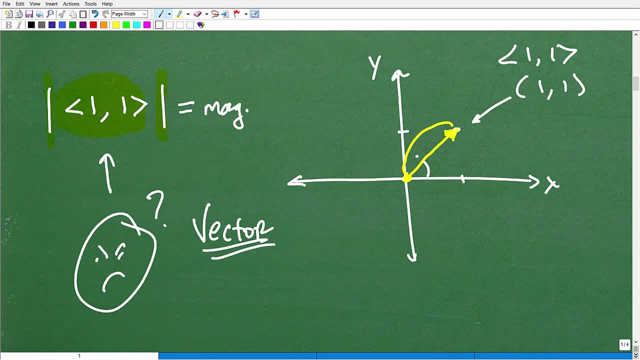 And this is certainly stuff that you, You're probably going to be doing in. you might do a little bit of an algebra 2, certainly in like precalculus, And vectors are everywhere. They're just hugely important. And this is the angle of the vector. 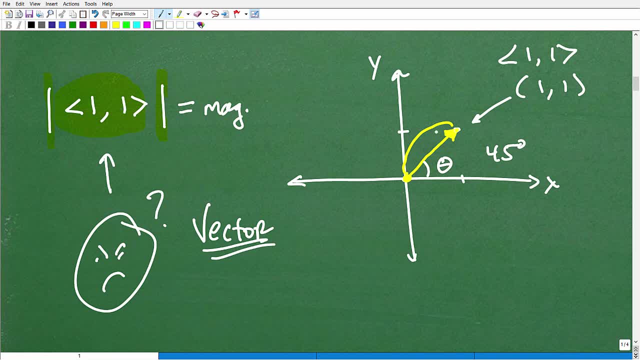 In this case, this would be 45 degrees. So how can I find the magnitude of this vector? Well, if this is 1 and this is 1, so I can use the Pythagorean theorem. Okay, So just like a squared plus b squared is equal to c squared. 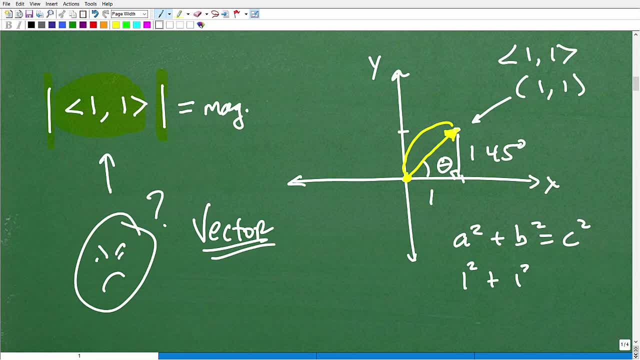 This is a little right triangle. So this is 1 squared plus 1 squared is equal to c squared. c squared Here, this is actually the magnitude of the vector, the length of that hypotenuse, of that right triangle. So we're going to get 1 squared, which is 1 plus 1, 1 squared. 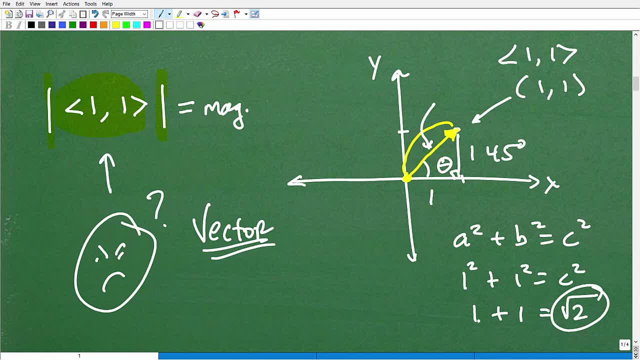 So that's going to be the square root of 2.. Okay, So well, let's just go ahead and do this problem properly. So c squared, c squared is equal to 2, c is equal to the square root of 2.. 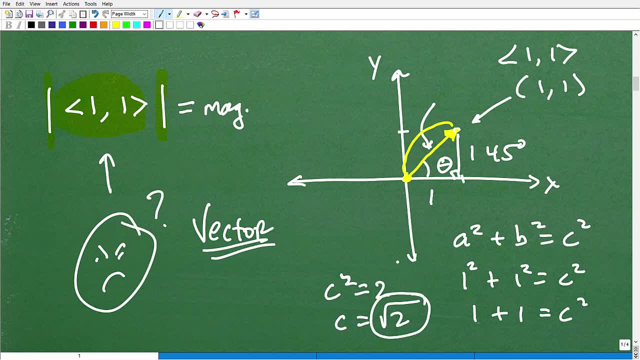 Again, we're only talking about a positive value right here. Okay, We're not going to, We're not going to deal with the negative 2.. So this is going to be positive. So the magnitude of this particular vector is the square root of 2.. 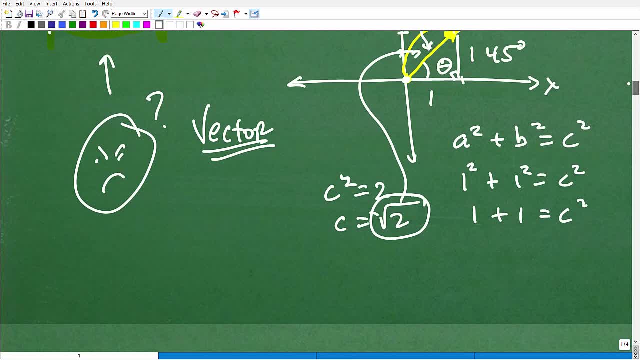 Now, if you knew this- okay, I you know, I'm going to have to change this right here- If you knew that that was the magnitude of the vector, if you knew all of these, then I must give you like an outstanding, crazy 1987.. 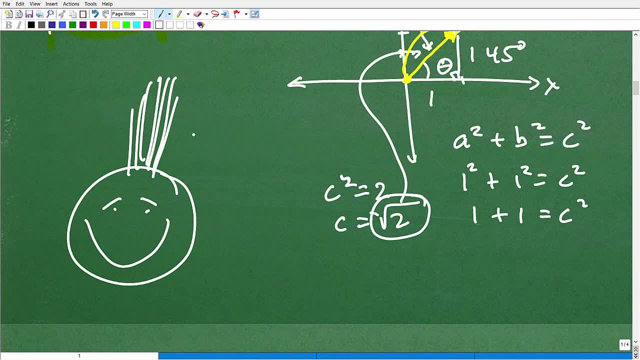 Now 1987, Mohawks were kind of going away, but maybe like 1987. Now 1985, yeah, that was a good year for Mohawks. So of course, if you've never lived in the decades, it was a pretty cool decade for sure. 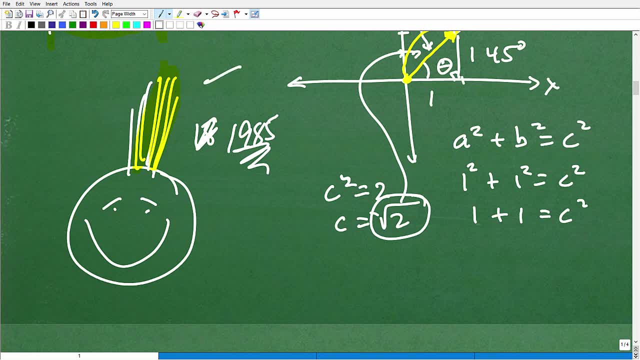 And we used a lot of hairspray because you know, people walked around with a lot of Mohawks back in those days. Okay, I didn't, I kind of sported this little flat top type of deal, But anyways, you definitely deserve an A plus a 100%. 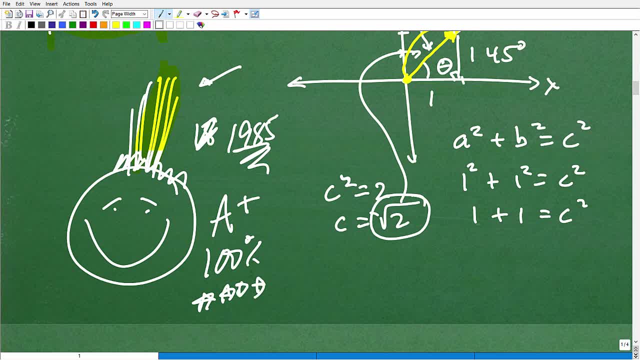 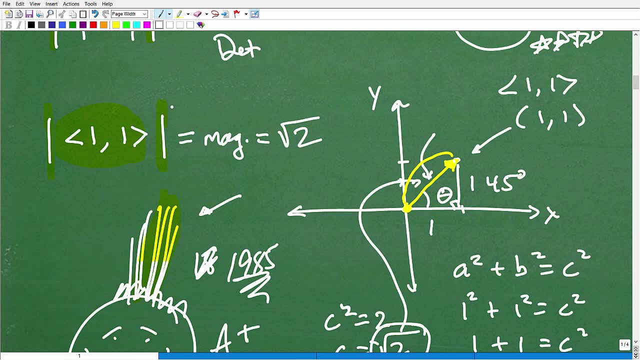 And I'll give you. let's say Now, although vectors is one of those things, you know, I don't think this is overly difficult. I mean, if you understood what I just did here, you know you understand this meaning. 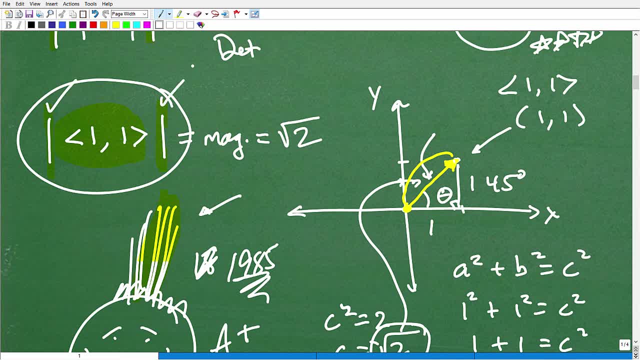 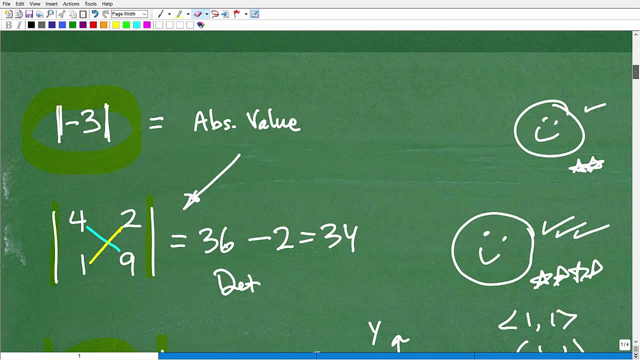 Okay, But what's the whole big point of this video? Well, you could have the same symbology, but it will represent different things. Okay, So you got to be paying attention to math. It goes back to what I'm talking about here with note taking. 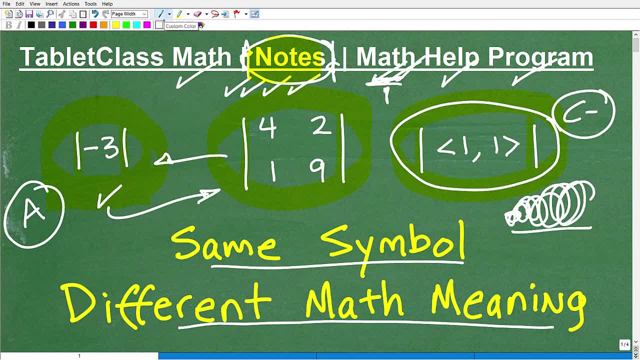 How could you possibly, you know, learn all this stuff and all the other stuff you're going to be learning without Really being engaged? Okay, So, if there was some sort of shortcut about learning mathematics, I would certainly, you know, tell you it. 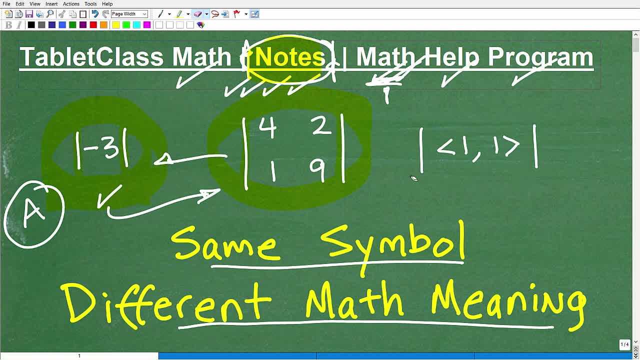 There's a little tricks and hacks and stuff. I try to share a lot of those on my YouTube channel. But anyways, if you found this little video interesting to some small degree, please consider smashing that like button. That definitely helps me out. 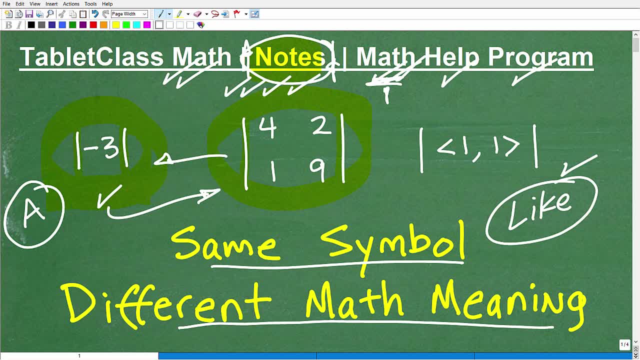 And if you're new to my YouTube channel, please consider subscribing. I've been on YouTube for 10 plus years, have over a thousand math videos, basic to advanced. I'm on my channel, So my goal is to try to make math interesting, clear and understandable.